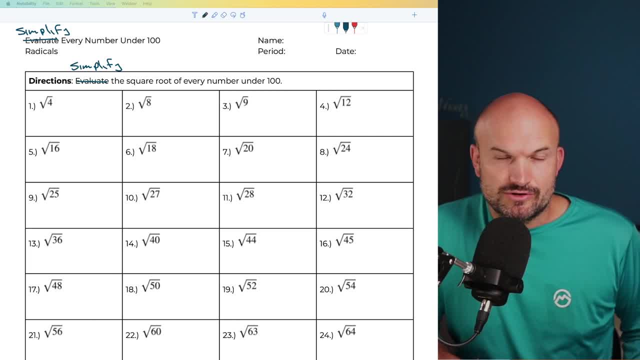 these problems. So therefore we can do this rather quickly. So the first one is going to be a square number, So that one's going to be rather easy. So the square root of four is just going to be a two. The next one, what I want to do, is square root of eight. I want to rewrite this. 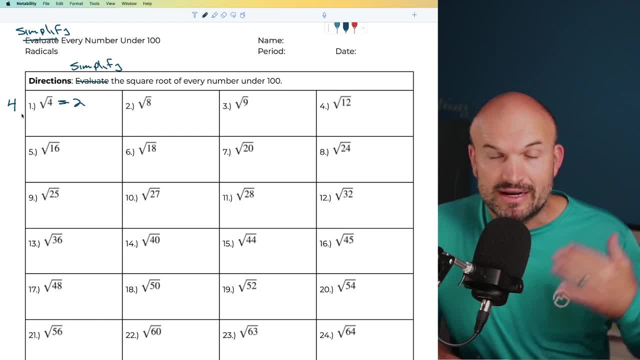 in terms of square numbers. So remember four is a square number right, Because you can take the square root of four. So I noticed that eight can be rewritten here as a square root of four times two. Now what I recognize here is I can take the square root of four, which is going to be two. 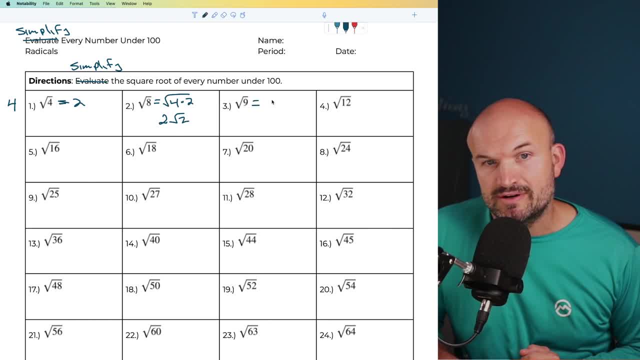 times the square root of two. Now, the next square number that we're going to have here is a square root of nine, which is going to give us a three. So I'm just going to write: nine is going to be another square number, Now 12, let's say that's not a square number. I can't take the square root. 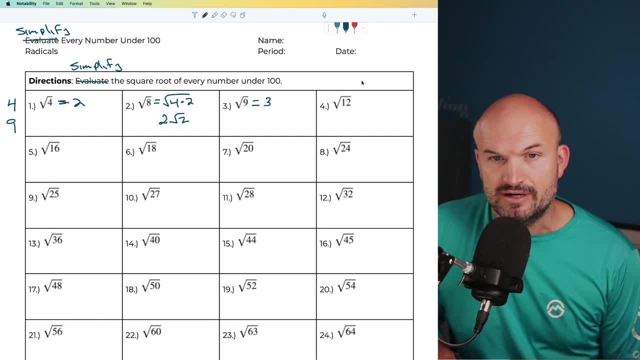 of 12.. But can I rewrite that as a product of my two square numbers over here? And yeah, you could say that's going to be a four times three. So therefore I can say: now this is going to be a four times three. I can take the square root of four, which is now going to: 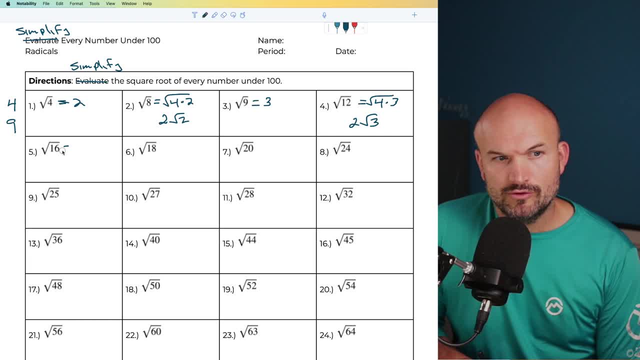 leave me to a two square root of three. The next one here- hopefully you recognize that as a square number- that is going to be a four. So that is going to be the next square number that I'm going to write out, Then the next one, eight. we would say: all right, which of these square numbers can 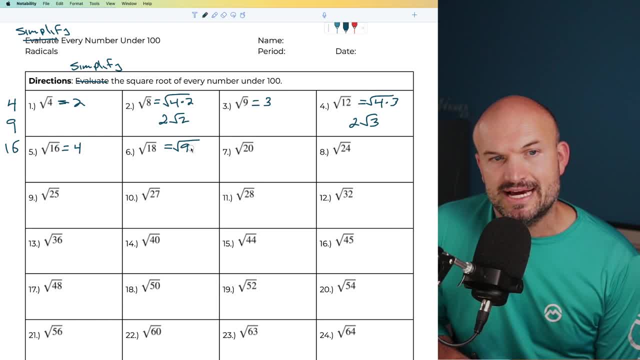 I rewrite that as a product And you could see that hopefully, that is going to be a nine times three square to nine is going to be a three square root of three square to 20.. I can rewrite that as a square root of four times five. Now, the one thing I want you to notice is- I'm always trying- 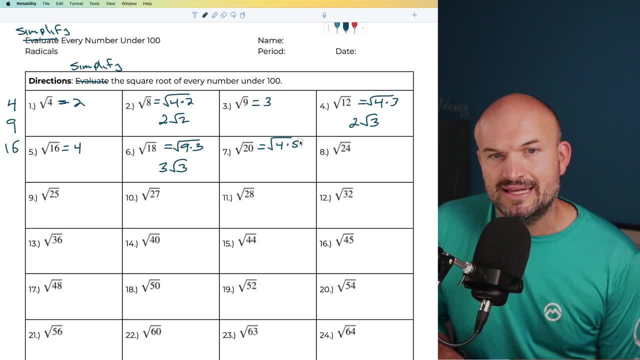 to write this square number first. You don't have to do that, but in my opinion I like to kind of always try to try to do that first, just to try to remain consistent. So the square root of four is going to be a two square root of five for the square root of 24.. Let's see, that looks like. 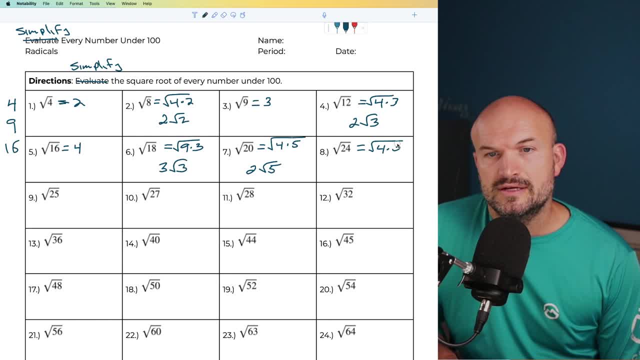 that's going to be a four times six. So I can rewrite that as a four times six And therefore that's going to be a two square root of six, the square root of 25.. That's going to be another square number, So that's going to be five. So I'll say: all right, that's another square number here. 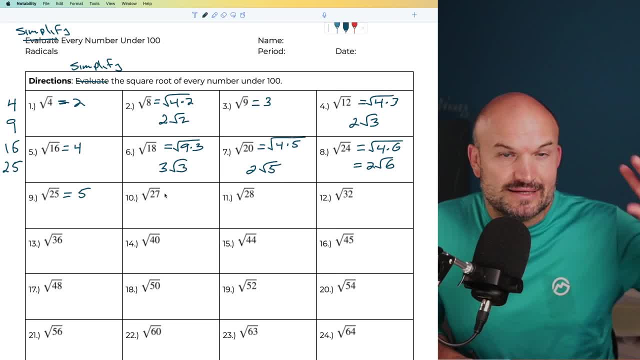 25 for 27.. Notice, a lot of times when they end in odd, you're going to be thinking of the nine, right, Because nine is my odd square number here, So therefore I can rewrite that as a square root of nine times three. I can take the square root of nine, right, Because that's a square number. 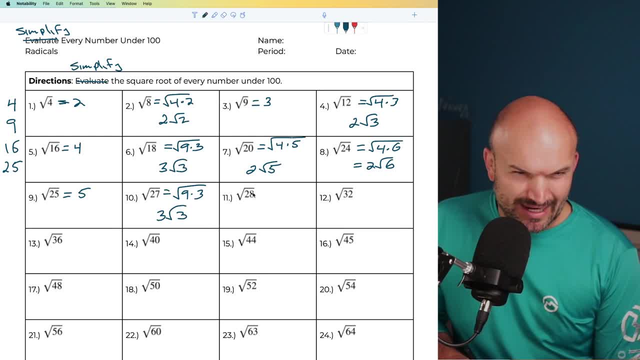 So, therefore, that's going to be three square root of three For 28,. it looks like that's going to be a four times a seven, right? So four times seven square root of four is going to be a two, And then I just have to leave the square root of seven under the radical right, Because you can't. 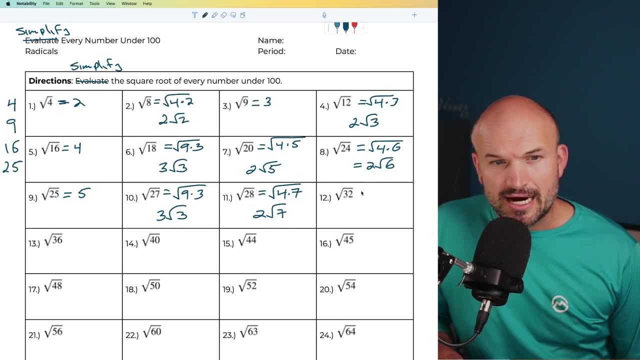 do anything with it. So therefore, you have to leave it there For the next one. here we have, and you could say: well, this is four times eight, right? But you can also say: this is 16 times two. So which one do you choose? Well, technically you can get to the right answer: choosing both. 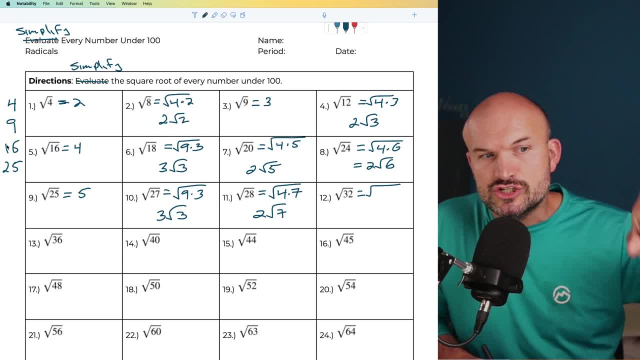 But I always like to do it. the way that I tell my students is always: choose the largest square number to rewrite as your product. So, rather than doing four times eight, I'm going to write this as a 16 times two. The square root of 16 is going to be a four square root of two. It just makes life. 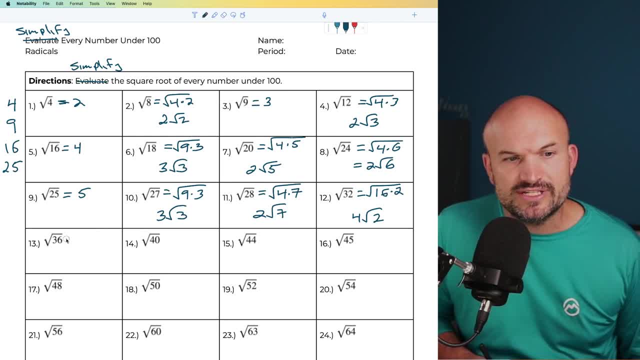 a little bit easier, And so, therefore, you don't have to do as much work. Square root of 36 is a square number. That's going to be six, So I'll go ahead and list this over here. Square root of 40. 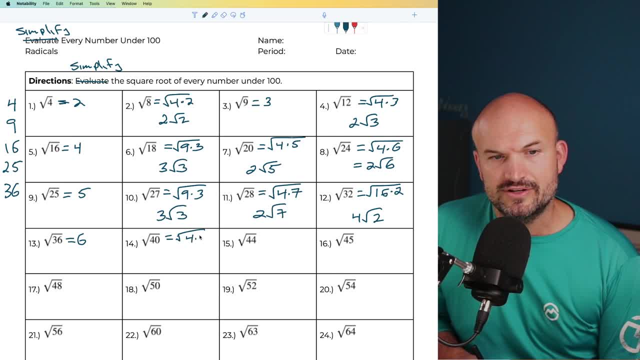 a square root of four times 10,. right, You can just rewrite it in that regard. Then I could take the square root of four and the square root of 10.. So, therefore, it's going to be two. Square root of 10 is my final answer For 44,. it looks like I could do a four times 11.. The square root of four. 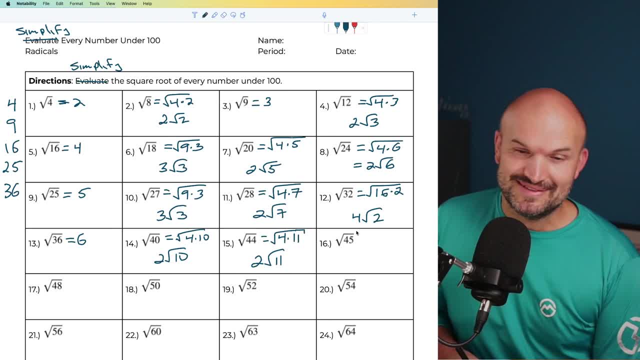 is going to be two, And then we have 11.. You can see we're using four, quite a bit right. So again, as you get through this, like the better and better you're going to get, Let's see 45.. I think that's. 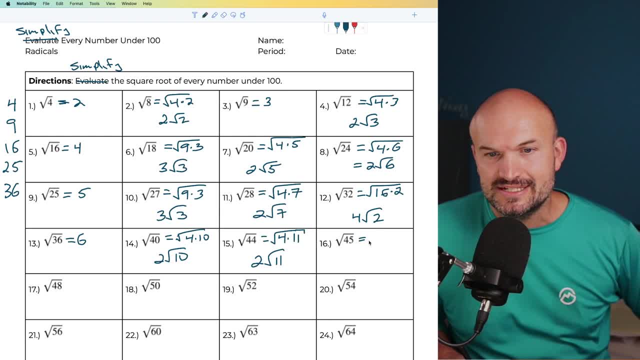 an odd number that makes me think of three or of nine, And indeed that is going to work. It's going on: a nine times five Square root of nine is going to be three times the square root of five: 48,. again, initially I think of four, right, Because it ends in an eight, but then I also. 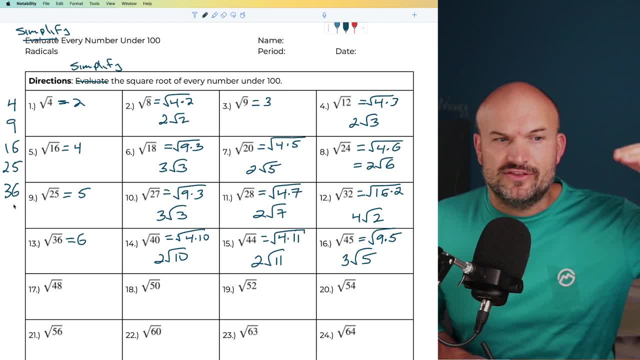 think is there a larger number right, And again, sometimes you can work your way backwards, like 36.. No, that doesn't go. 25,, no 16.. Ah, 16 does work right. So again, sometimes you might. 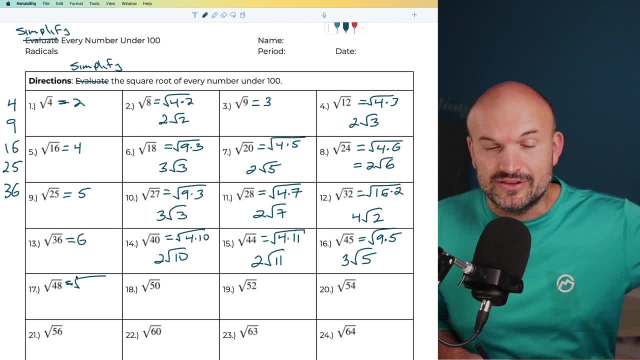 have that initial thing like: oh, four is usually going to go into it, but is there a number higher than four, a square number that evenly divides into that? In this case we do have. we have a 16 times a three. Square root of 16 is going to be a four times square root of three. 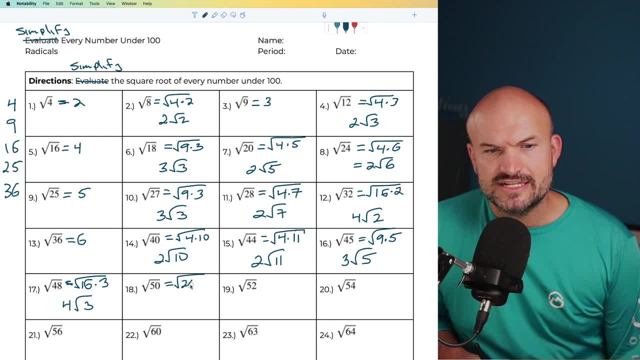 Here 25, I know is going to 50, or I can rewrite that as a 25 times two Square root of 25 is going to be a five square root of two. And then for this one here now, this one, you can start kind. 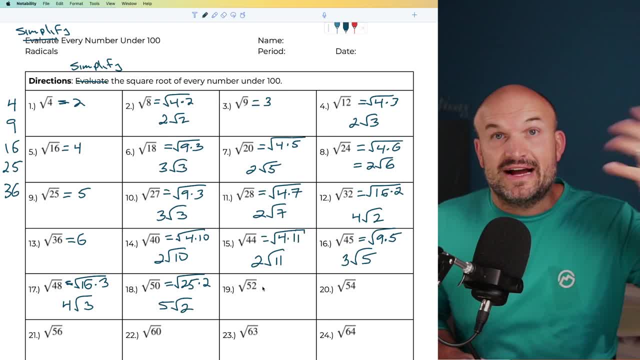 of taking with like number 19.. What you can do is like start thinking of this as like dividing it by two right, That's an even number. So if you divide it by two right, that's going to be a 26. 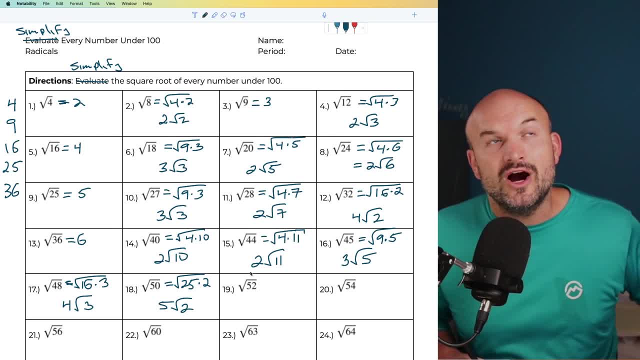 divided by two, Again, that's going to be a 13.. Oh, 13 times four, right? Because you divided it by two, which is technically divided it by two, Which is kind of like dividing it by four. So, even if you don't know initially, like how many times, 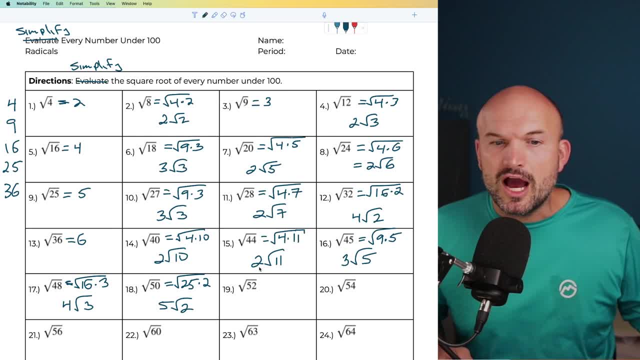 is four going to 52, just keep on dividing it by two, That's, and then you'll see like, oh, two went. divided by two twice was same thing as divide by four. So therefore I can rewrite this as a four times a 13, and square root of four is going to be a two times a square root of 13.. 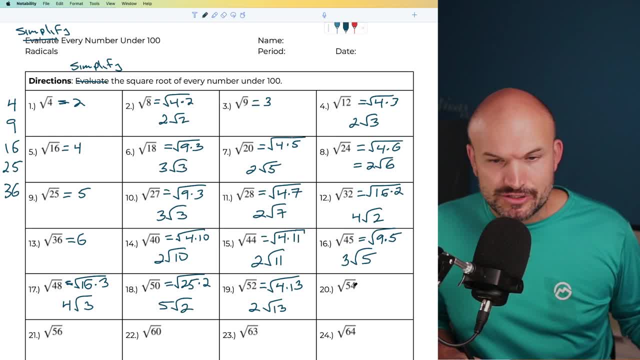 The next one over here, this one's even, but again, hopefully you recognize, you know your multiples are nine, You recognize. oh, this would be nine times a six. So I have a nine times a six. So therefore that's going to be a three square root of six. Okay, Again the same thing. 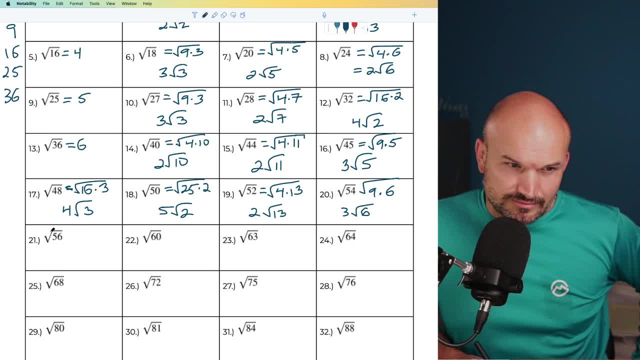 I'm going to do over here. I'm going to divide this. Let's see: if you divide this by two, that is going to be a 28, divided by two Again, that's going to be a 14, right, And 14 cannot be simplified. 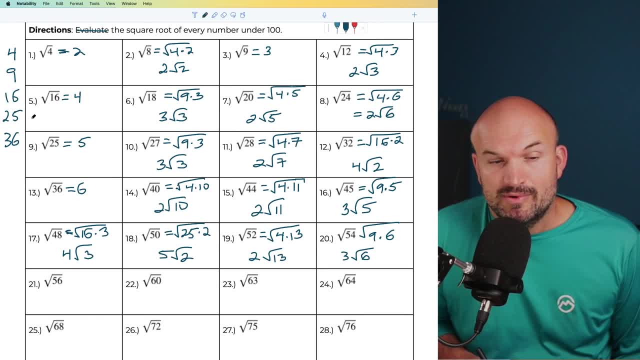 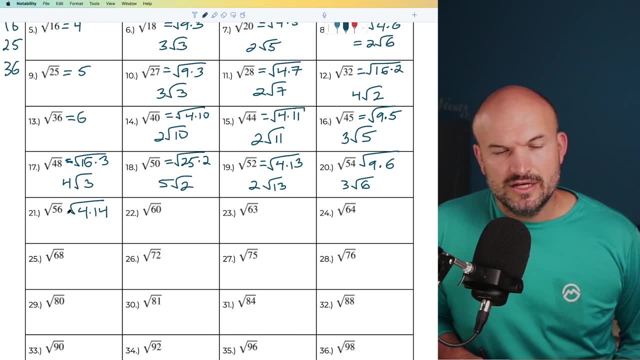 any further. There's no other square numbers that you can divide into a 14.. So therefore, that is going to be the next one. So let's see, I can rewrite that as a four times a 14. square to four is going to be a two. 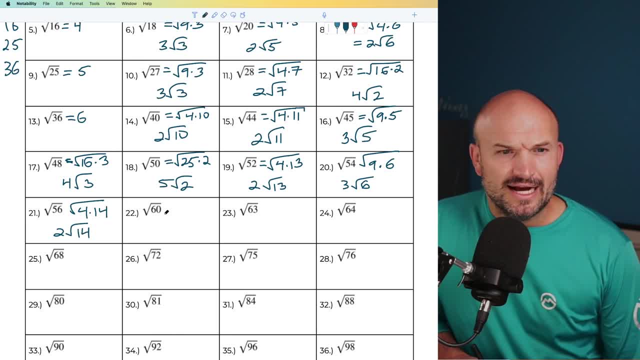 Square root of a 14.. Again 15,. hopefully you recognize 15,, 60 or, or, I'm sorry, going again through this, I recognize that 15 divided by 30, divided by two, again it's going to be 15.. 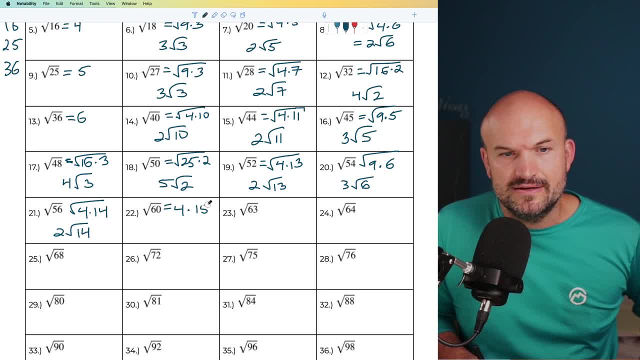 So therefore, I can rewrite this as a four times a 15, and square root of four is going to be two times the square root of 15.. Now here I recognize an odd and I say: oh yeah, nine, does nine go into 63?? Oh yeah, Seven times, right, Or yeah, seven times. So therefore, I can rewrite this as a nine. 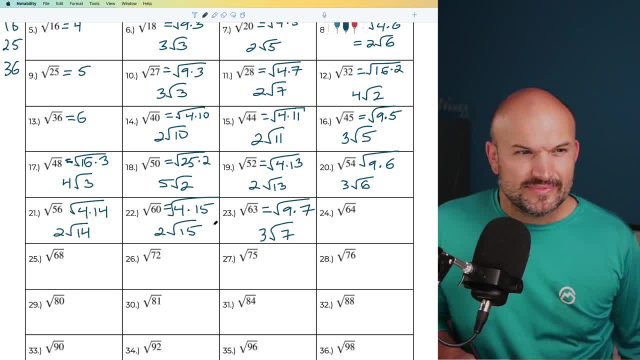 times a seven square root of nine is going to be a three square to seven. Um, did I miss a couple? I think I did 36.. Where did I get to? Oh my God, I did forget 49.. Holy crap, Let's go ahead and do. 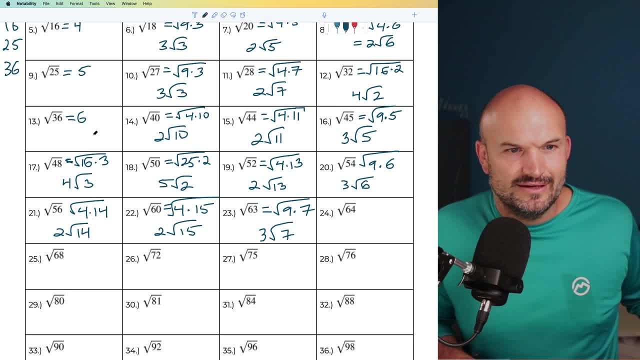 I was wondering about that. I'm like: where'd 49 go? So I forgot to type that in Shoot. Okay, Well, let's go ahead and add 49.. Then there's a 49 that goes into there, guys. So square root of 49.. I must. 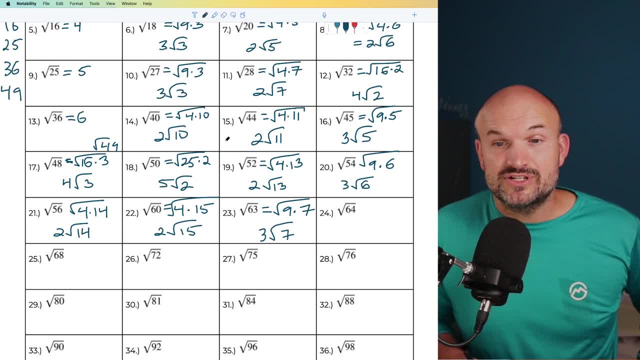 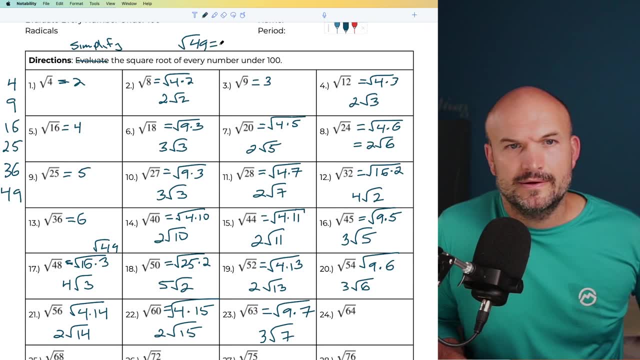 have missed that square number. So we have 36 and we have 49, which is another square number, right? Because, um, let me go ahead and write that up, Um, square root of 49 is going to equal seven, So I will update the sheet for those of you that. 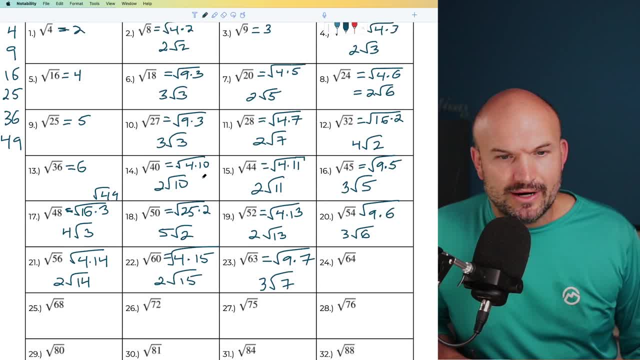 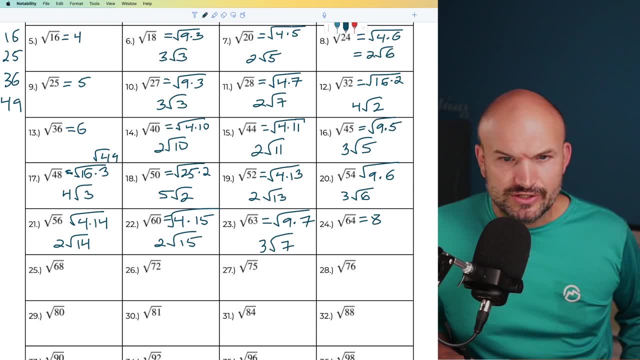 are following along from that. I can't believe I forgot about that Um. all right, So, and then we have square root of 64, which is going to be an eight Um, and then let's go and get into. 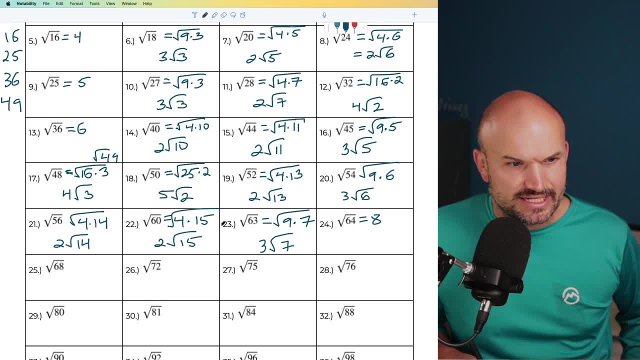 okay, So now we have 25, which is going to be a 68. Okay, So, again, we divide by two. um, it's 34 divided by two, Again, it's going to be a 17.. So you could say: all right, so let's say four. 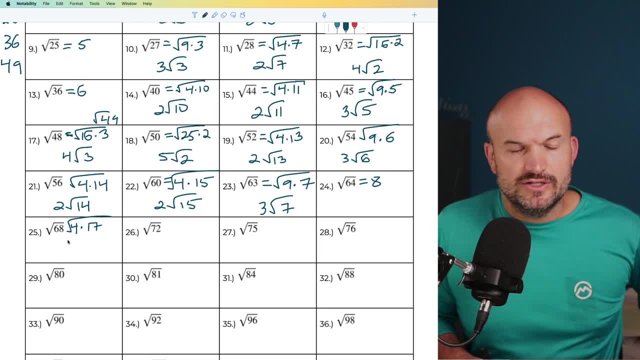 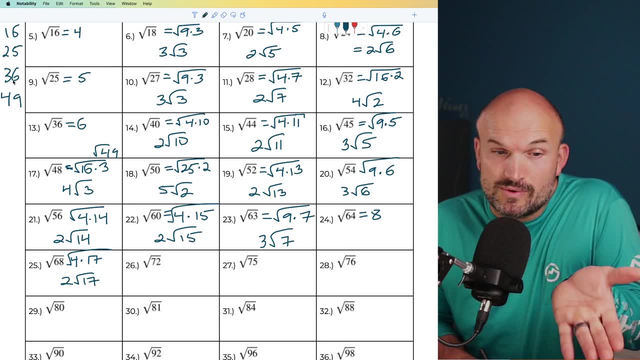 times A 17 square to four is going to be two times a square to 17. here I recognize um again, divided by two is a 36, right, Oh, 36 is a square number, So I can rewrite this here as a 36 times. 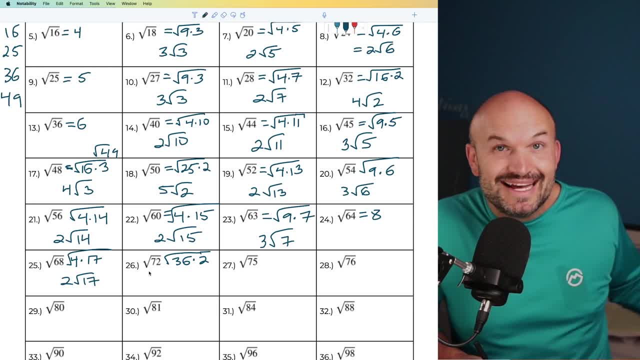 two. A lot of people might say, Oh, can't you do nine times eight? Yes, of course you can, Right, But again, guys, our goal is to do the largest number, largest square number that evenly divides into that term Um. so therefore, we have a um 36.. Well, that's going to be a six times. 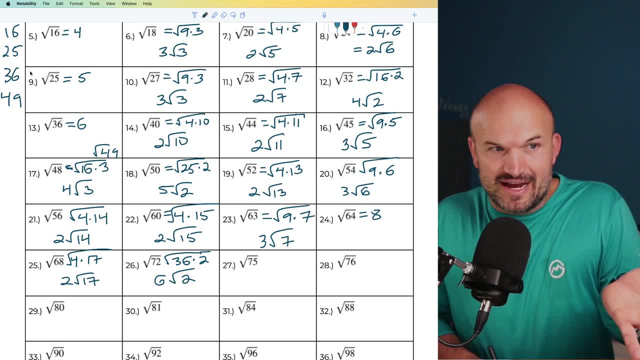 So square root of two. here I recognize a ends in a five: 75,. 25 goes into there three times, So I can rewrite this as a 25 times three, square to 25.. It's going to be a five times a square root. 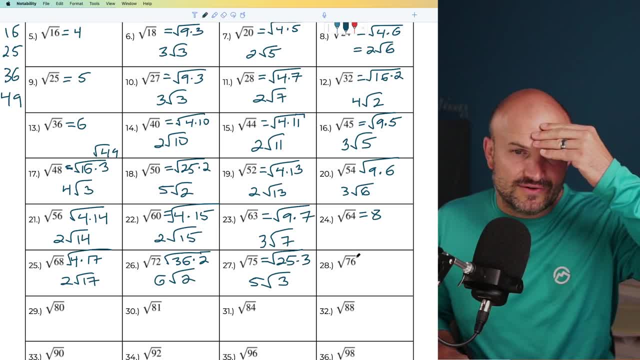 of um three And then this one. I'm going to divide out Um. I'm not sure what 76 starts to get big numbers right, But I know it's even so. I can divide it by two. um divided by two. 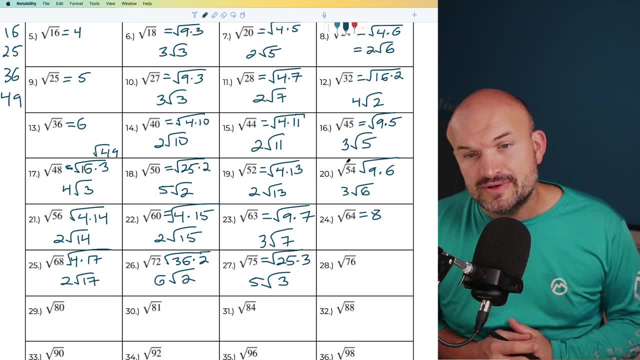 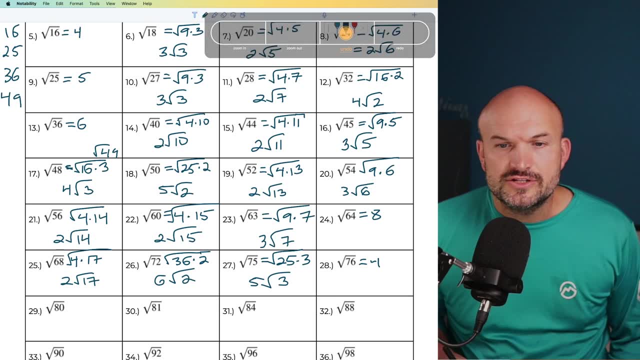 That's going to give me a 38,. uh, divide that by two. Again, that's going to be 19.. I'd say, Oh, okay, So I can rewrite this as a four times Nope, Let me just fix that up. So this could be a four times a 19.. 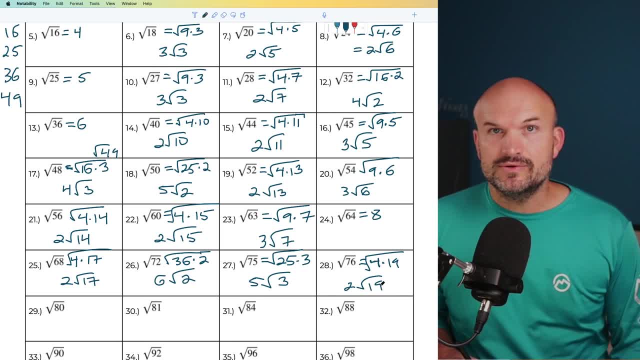 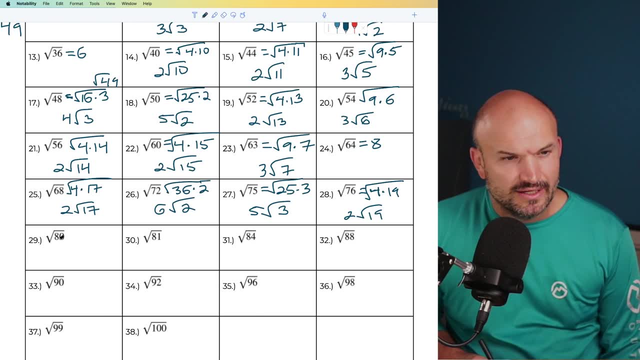 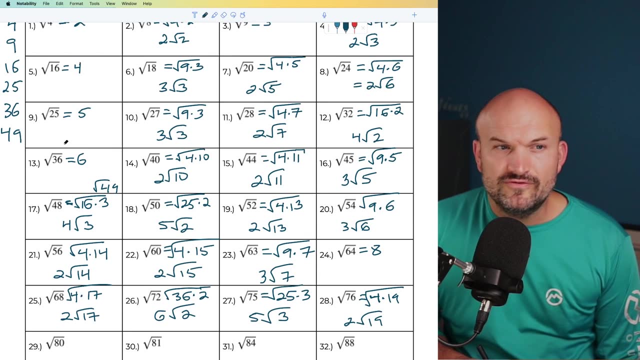 There you go, And the square root of four is going to be two times a square root of 19.. All right, Now let's go and get into our 80, which is going to be: um, let's see here. So, thinking of 80,, um, I recognize that, let's see here. And now I know four is going to go. 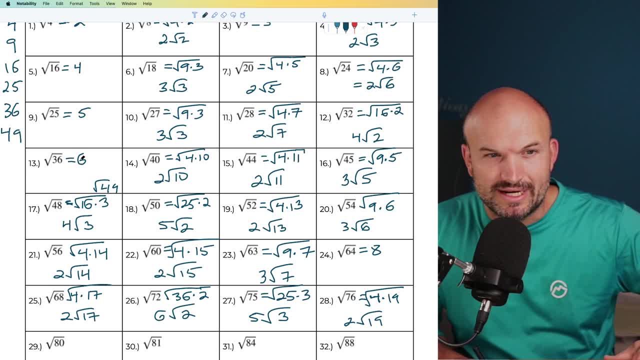 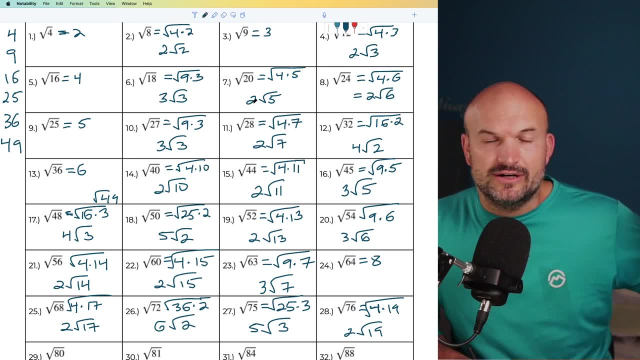 into there 20 times, right, But then I can reduce square root of 20,, right? If I think about square root of 20, that's going to be um, a two times five. So that'd be already. you're going to be multiplying the ends, Um, so then the two times four, which is going to give. 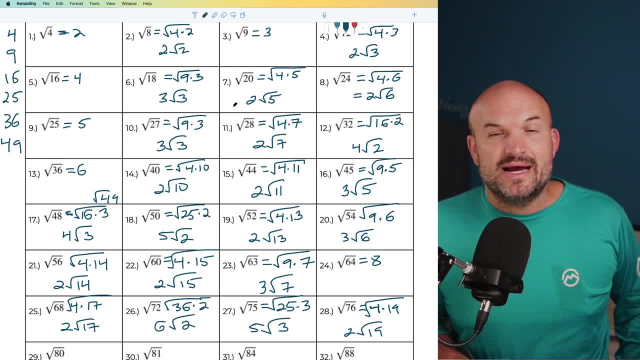 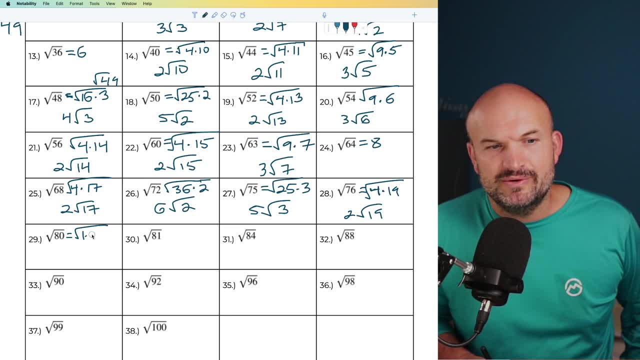 you, or two times um two, which would give you four. So I'm actually giving your final answer is four times square root of five. but let's see that means what this is. So I'm kind of doing my mental math in my head. This can be rewritten as six. How many times is five going to there? 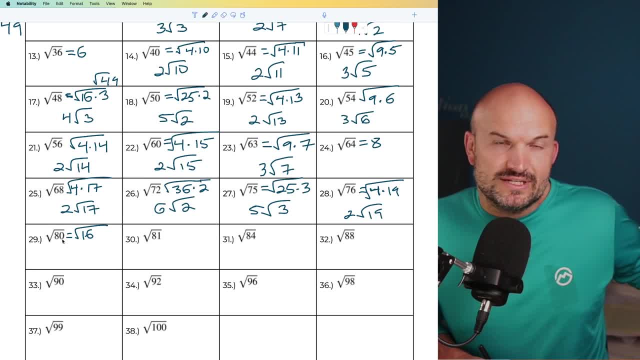 Well, that's going to be: five goes into 50, 10 times, and then it's going to go in there four times. Um, yeah, 10 times, And then, I'm sorry, there's an extra 30.. So that'd be. 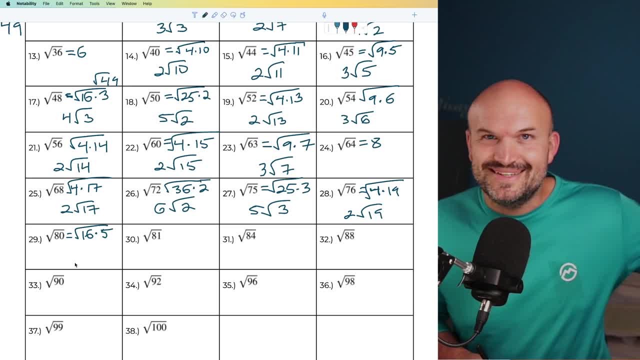 there we go. So 16 times five. doing some mental math in my head, Don't bother me. Square root of 16 is going to be a four square root to five. I'm sure none of you have tried like doing all of these problems all at once Like it's such a great idea. Um, oh, man, Okay. 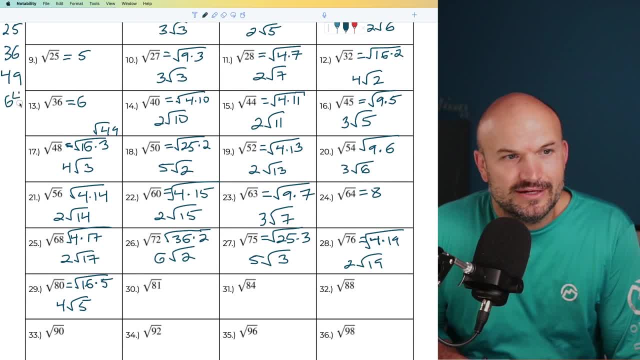 Ooh, And the next square number. why did I keep my friend? So we have 64.. That was a square root of eight. I forgot to write that in there. Sorry about that. The next one: we have nine, right, So? 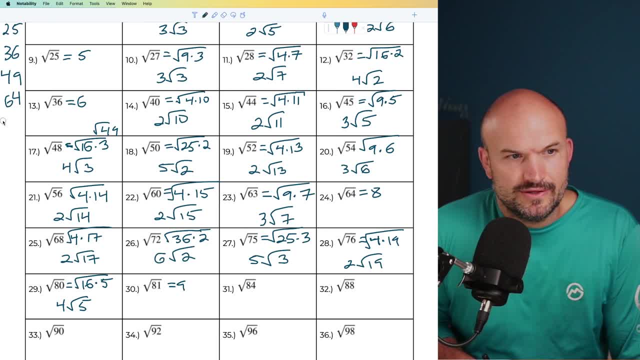 square root of 81 is going to be a nine, So that's going to be 81, which is our next square number. Um, then we have our, our 84.. So okay, So let's divide that by two. Um, that's going to be a 42 divided by two Again. 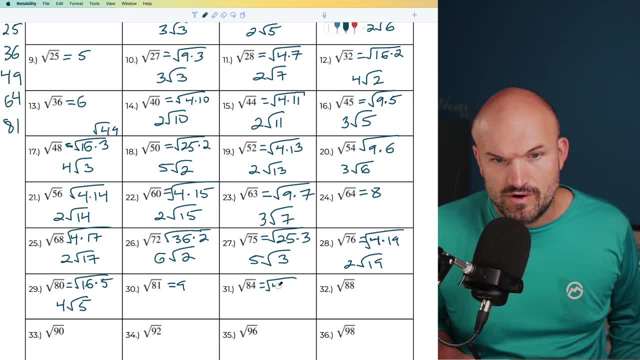 that's going to be a 21.. So, therefore, I can get that. as to a four times a 21, square to four is going to be a two times a square root of 21.. Then we have a 32.. Um, again, we can do the same thing. 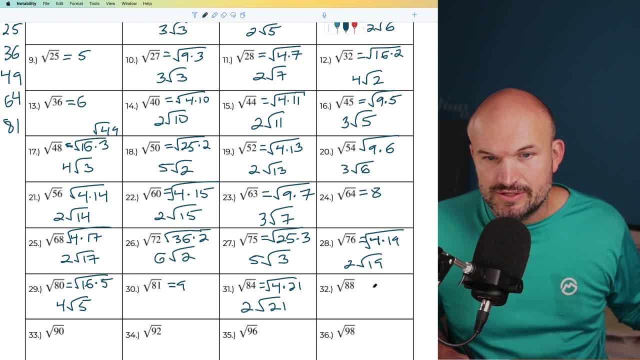 divided by two is going to be a 44. divided by two, Again, it's going to be a 22,. right? So therefore I can do a four times a 22.. So notice, if I don't know exactly, there's already a bigger number. 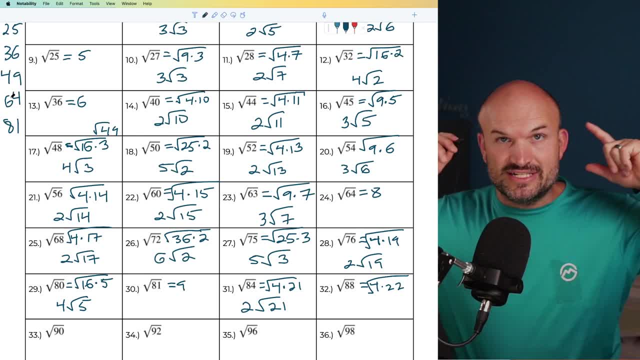 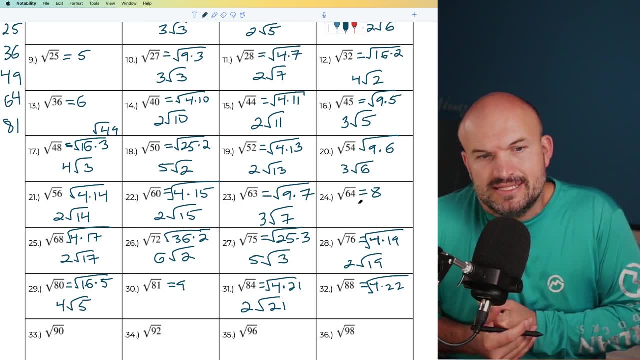 that knows evenly into it. I kind of work with my prime factorization to divide it by two, um, to kind of see what is going to work. And a lot of times, if anything else doesn't work from that case, then I'll just, you know, divide by two in that case, to see what I can do. 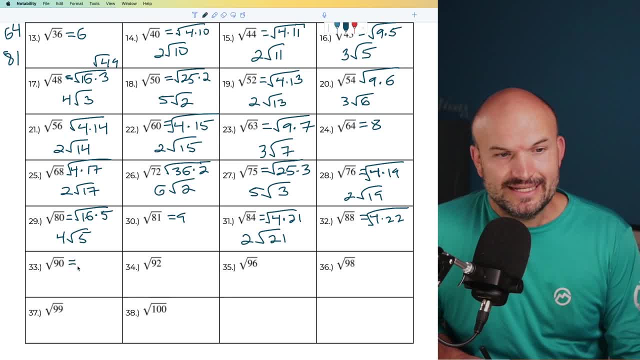 Um, all right. So nine times 10, well, I know, nine obviously 90.. So that one's going to be a nine times 10 square root of nine is going to be a three square root of 10.. Um, now this one. 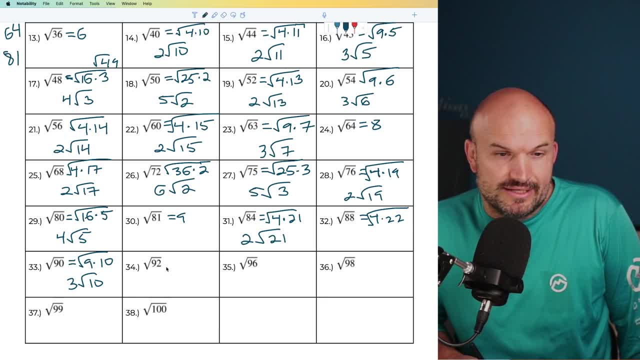 could be a little bit of interesting here. So, um, it's even right. So let's see that would be a 46. And then if I divide a 46 again, that'd be a 23. So again, I'm just 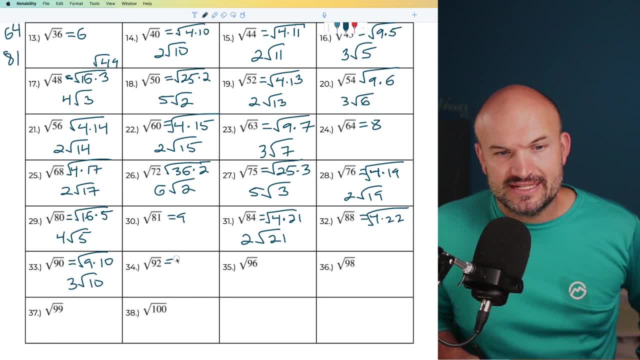 divided by two, twice, which is technically divided by four. So therefore I can say that's the same thing as a four times a square root of 23.. Um, oops, I'm sorry. Let me fix that correctly. You're rewriting it under the radical as a four times a 23,, and then square root of four is going. 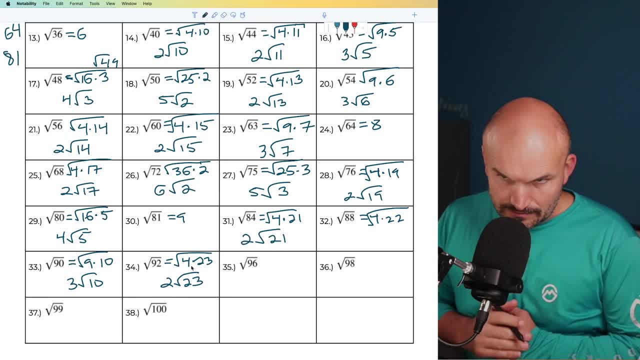 to be a two times the square root of 23.. All right, Now we have our 96.. Um, which, again I'm thinking into this one, like I don't think I need to divide by four. 96 sounds like a pretty common number And again, if I'm thinking about, 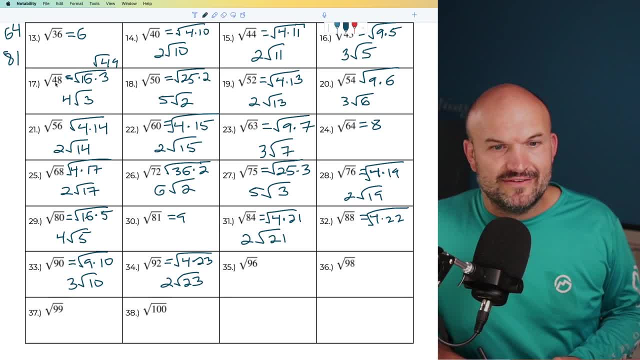 96,. um, that was already half right of 48. And I know 48 can be divisible here. So what I'm looking into is saying: all right, well, that's going to be. what else can I simplify there? So that one 16 went into there three times. So if it's not double, 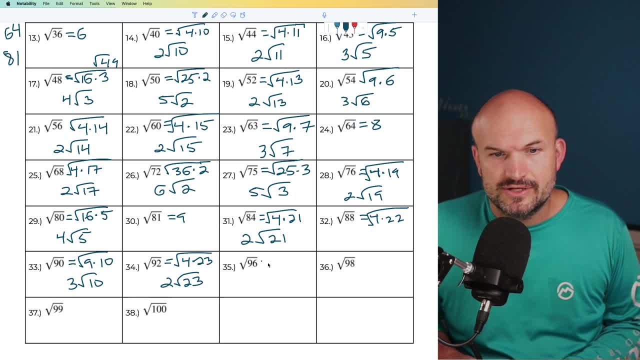 that means this could be written as 16 times a three times right, So therefore I can re: I'm sorry, 16 times six, So therefore I can write this as a 16 times six. square root of 16 is going to be a four square root of six, um 98.. 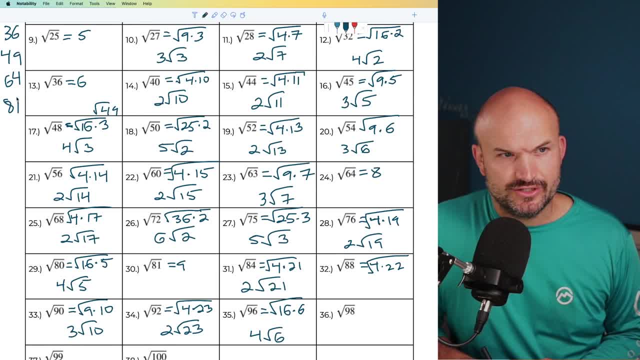 Hmm, Uh, let's go and see if we can do a square number here. What if I double 49? die too right, That's getting to be 98.. So that one's kind of actually easy. So therefore I can rewrite this: 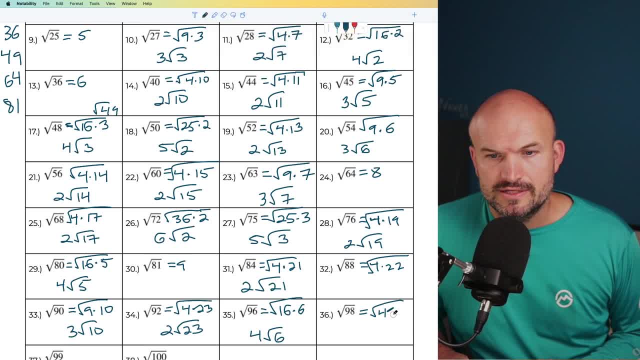 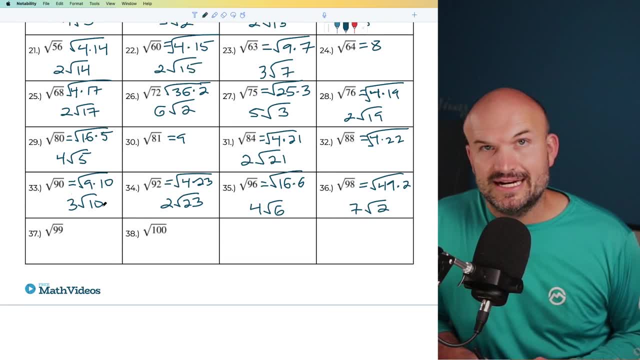 as a 49.. Come on, write your 49s correctly. It's supposed to be a 49 times two. square to 49 is going to be a seven square root of two, Um and 99, that's going to be a nine times 11.. That one's.